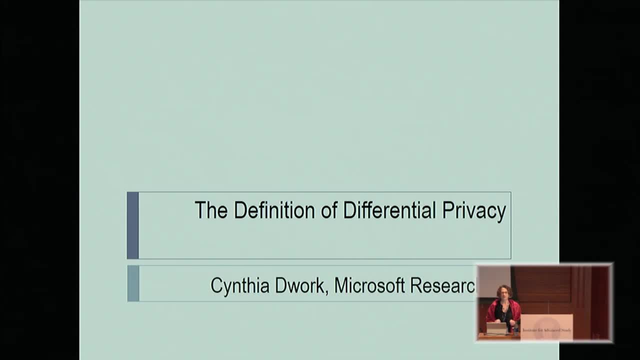 speakers to concentrate on their specific topics, And this definition is ten years old and this presentation of the definition reflects ten years of evolution in how to explain what's going on, Because from the formula itself it's not quite so clear. One of our speakers 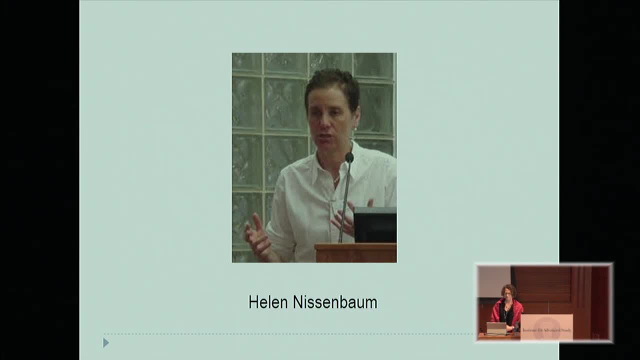 today is Helen Nissenbaum And in fact I got interested in working on privacy in general because of conversations that I had with Helen in about 2000 or 2001.. And I was looking for some because of my discussions with Helen. I was looking for some piece of the privacy. 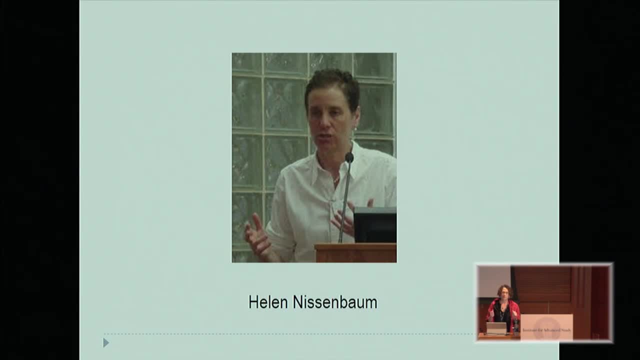 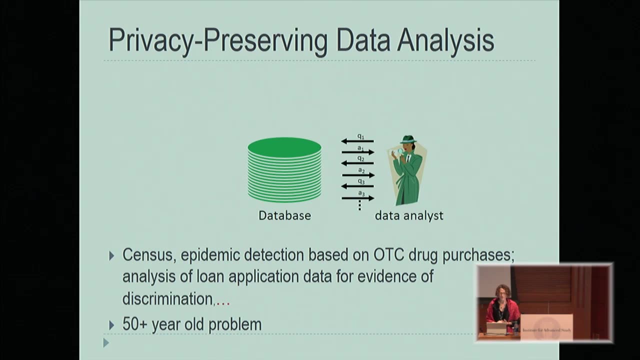 problem in general that we might be able to sort of tame with mathematical rigor, And we settled on. I settled on privacy-preserving data analysis, So the driving application or example that I had in mind. I was talking this over with my then-intern, Adam Smith- 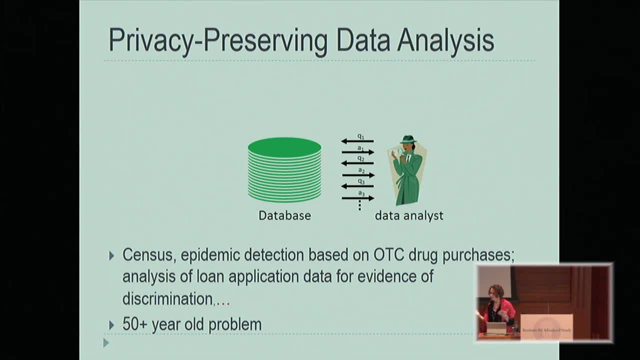 was the Census Bureau. The Census Bureau has the data of the people. It is being analyzed for the benefit of the people. It is being analyzed for the benefit of the people And the data, when you look at it, is in the form of an audit of the people to apportion the 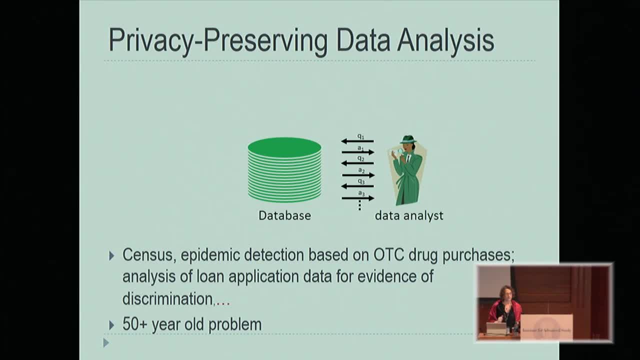 people's resources And there is a legal mandate for privacy. So how can you analyze data while preserving privacy was the general topic, But of course it goes way beyond Census. You could use it for epidemic detection based on over the counter drug purchases You'd. 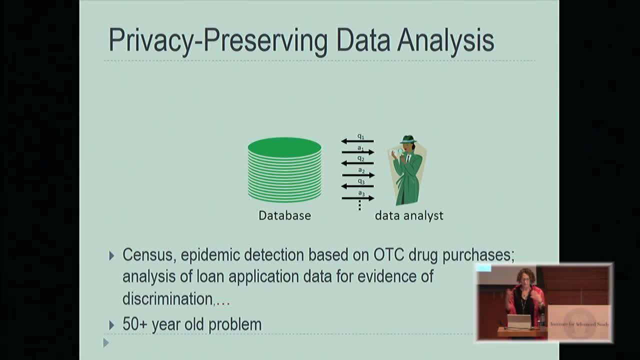 like to keep the individual purchases private, but you'd like to see that there's an epidemic happening: Analysis of loan application data for evidence of systematic discrimination and so on, And this question of how to analyze data while preserving privacy is a very old question. It's at least 50 years old in the literature. 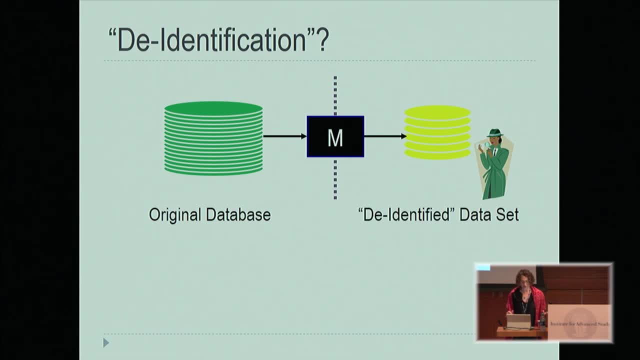 So one thing that many people think of is, well, just de-identify the data. So that means you start with some kind of original database, you pass it through some kind of mechanism or machine, M you reveal, maybe you delete some outliers and some fields and you release. 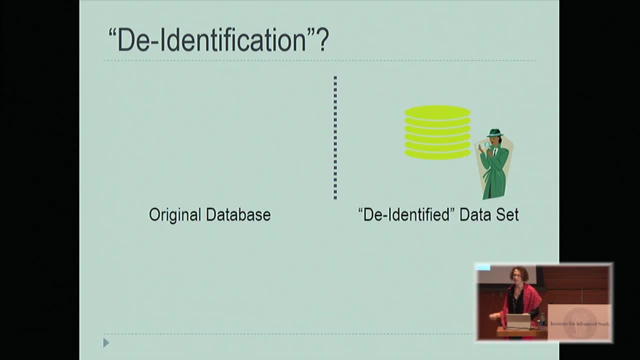 some kind of de-identified data set And you say to the data analyst: have at it, Find anything you want. Just look at this de-identified data And the only thing that we're going to say about that is that de-identified data isn't. 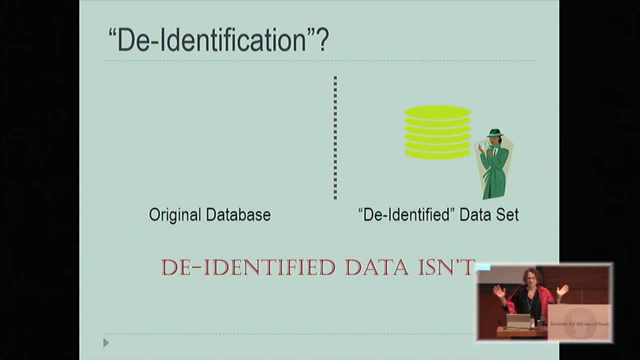 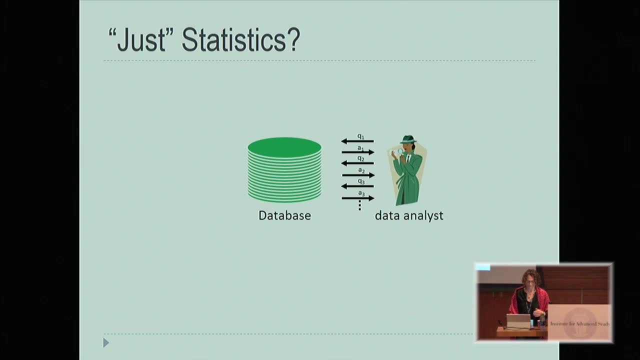 Either it isn't data or it isn't de-identified. So we're just not going there, And I can point you to many places to back up this statement. So the next idea is: well, you want to do to do statistical analysis of data, so just release the statistics. 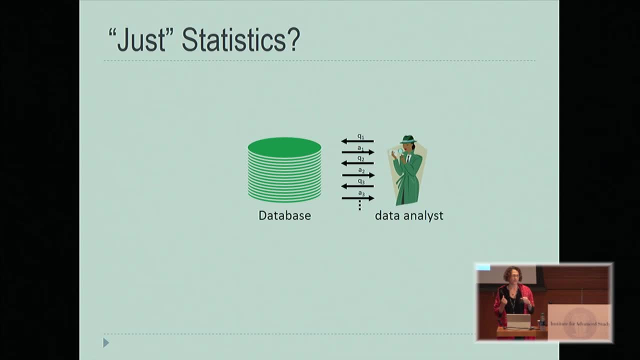 So in our imagination we have our data analyst. She asks a question. She asks for the number or the fraction of people that are over six feet tall and like donuts or things like that. She gets an answer. She asks another question. 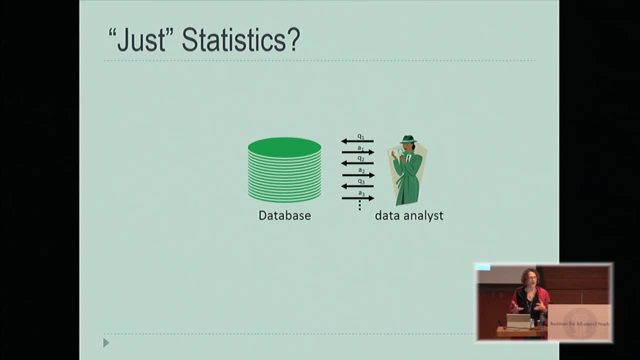 She gets an answer, And that's going to be our general model of how a data analyst who can't see raw data because that would be privacy disclosive, and who can't see even de-identified data because that doesn't work. 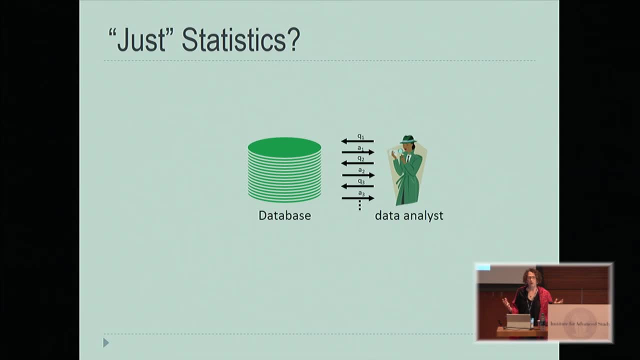 So she has to interact with the data set by asking questions. So what if we just give her statistics And your intuition says, hey, a statistic is, it's not going to be dramatically affected by the data of any individual. That's the whole point of a statistic. 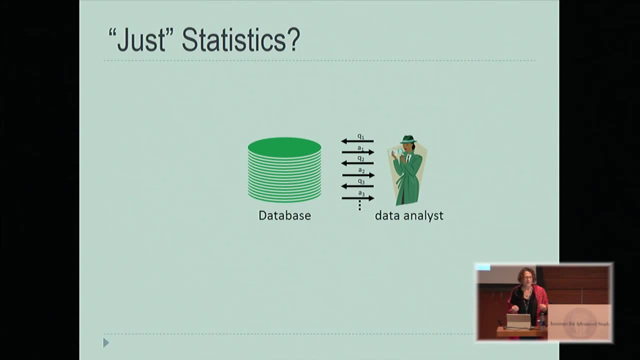 It's like you take, you know you compute some quantity from a sample and it shouldn't really matter. It doesn't matter which your sample is, Otherwise it isn't a very interesting statistic. It isn't an interesting measure of your population as a whole. 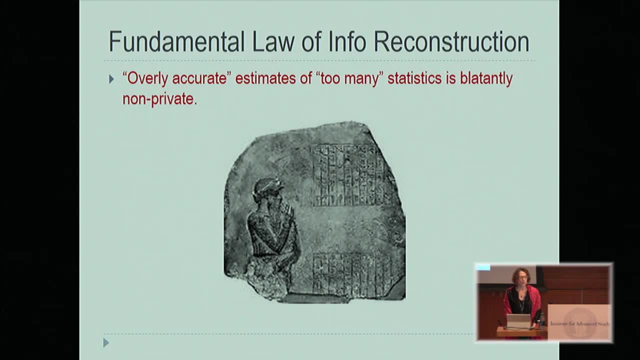 So, to make a long story short, there's a whole host of results that have now become known collectively as the fundamental law of information reconstruction, And they say, roughly speaking, that overly accurate estimates of too many statistics completely destroys privacy. And this will in fact be the subject will be touched on rather heavily, actually, by 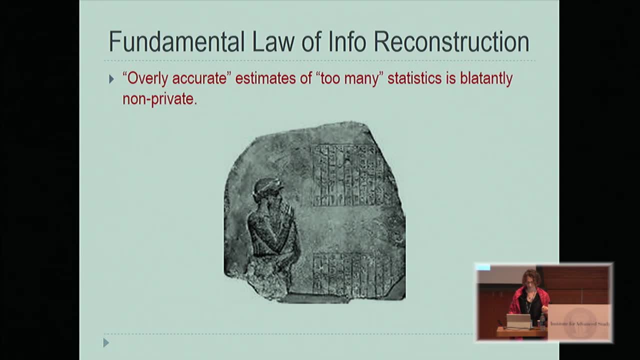 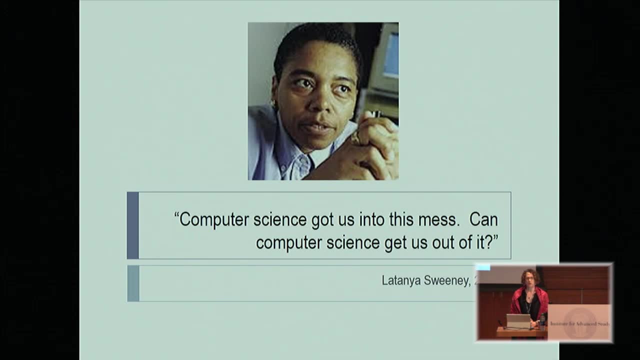 Jonathan Ullman in his talk Dusting for Fingerprints. So Latanya Sweeney, who is a master de-identifier, when she was the head of the, the CTO of the Federal Trade Commission, said: computer science got us into this mess. 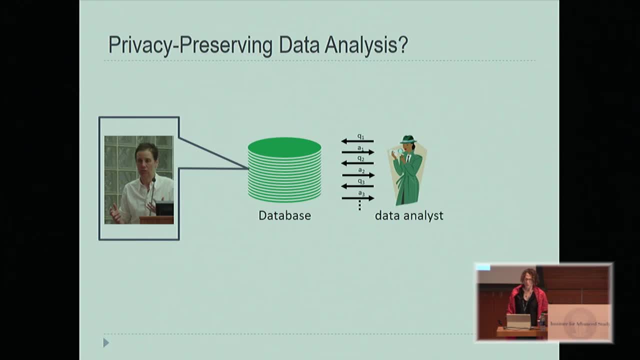 Can computer science get us out of it? So, with that in mind, how can we define what it is that we're trying to do? How can we define privacy for the purposes of privacy-preserving data analysis? So here's a data set. 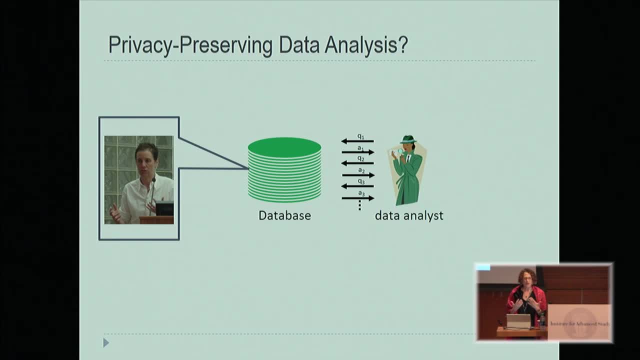 Helen Nissenbaum is in the data set. The question is, what kind of privacy, what kind of guarantee do we want to make to Helen? So the first thing that you would try- And in fact there's a lot, This intuition dates back in the statistics literature at least to Tord Delinius in 1977,. 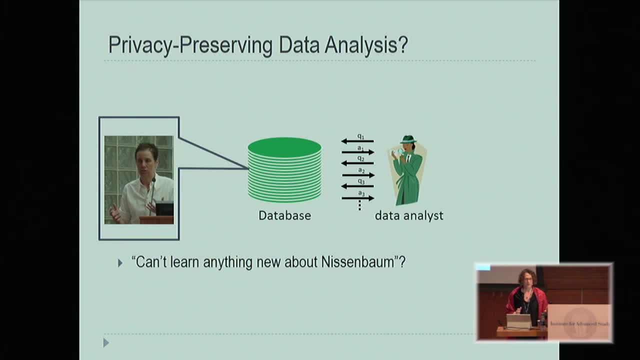 says that the data analyst, by interacting with the data set, shouldn't be able to learn anything new about Nissenbaum that the analyst didn't know before having access to this data set. So Helen may have a website where she has all kinds of information about herself. 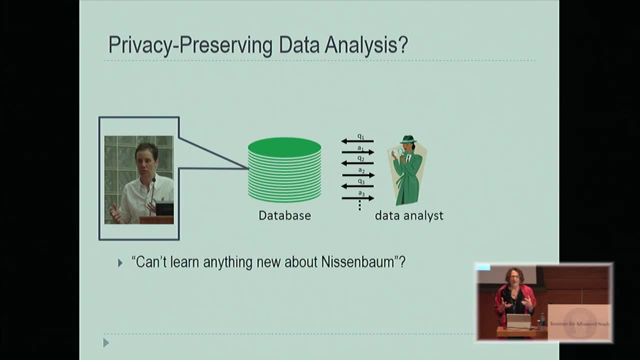 Anybody can know those things because she's posted them, And the fact that she's posted them, And the fact that she's posted them, And the fact that somebody would know them, is certainly something you can't blame on this statistical database, because Helen posted them. 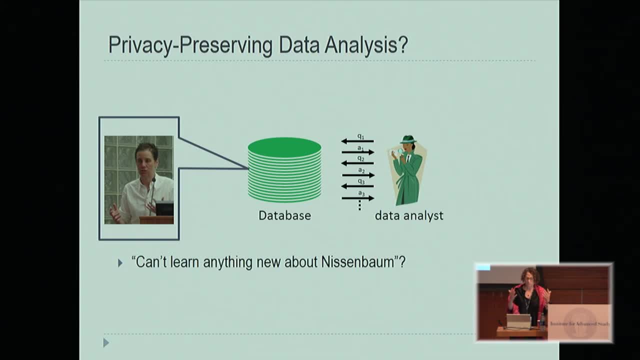 But maybe you want to say that we shouldn't learn anything new about Helen, that she didn't post about herself, And the problem with this definition is basically what is the point? So we do statistical analysis of data because we want to learn something about the population. 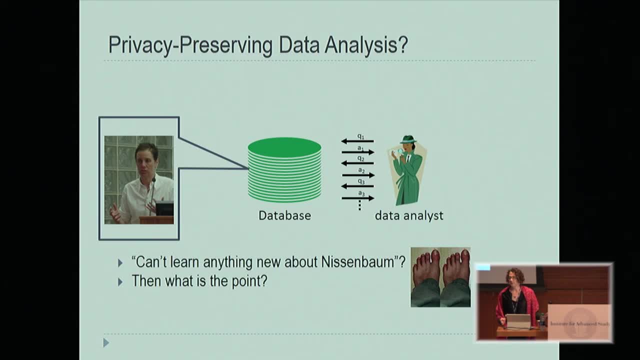 Let's suppose that I'm from Mars and I believe that all humans have two left feet. So, in particular, I think that Nissenbaum has two left feet And I analyze the data set and I learn that almost all humans have one left foot and one. 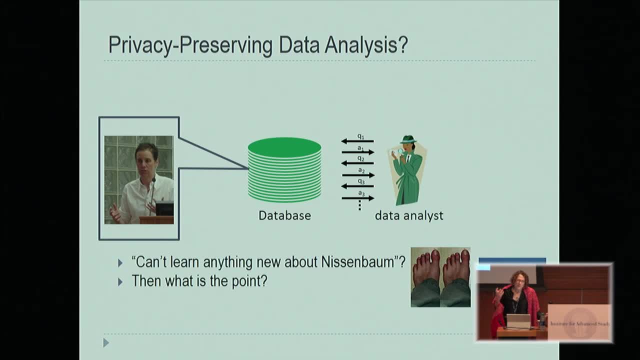 right foot. So my beliefs about Helen have changed. I now think she has one left foot and one right foot. I learned something new about her And the question is: did I compromise her privacy or not? Now the question is: did I compromise her privacy or not? 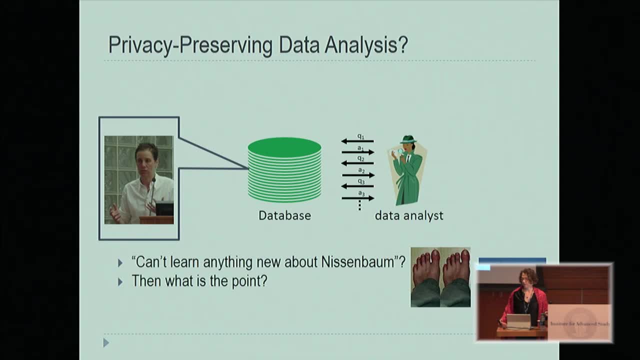 Now the question is: did I compromise her privacy or not? That's a definitional choice that we make. Do we want to call this a privacy compromise? We learned something new about her, So we took the position that, no, this is not a privacy compromise. 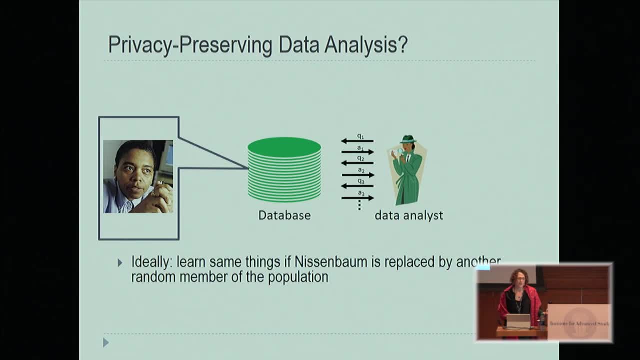 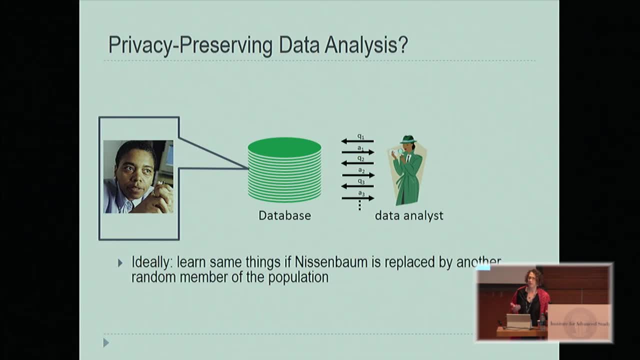 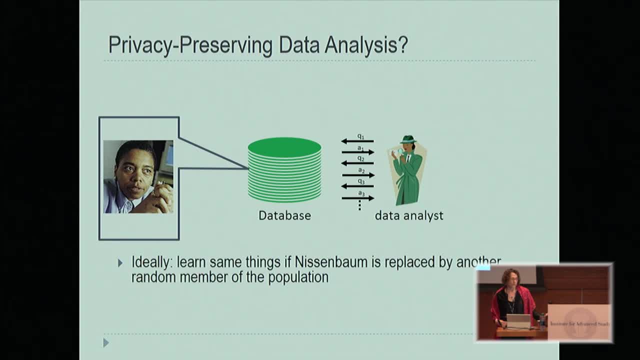 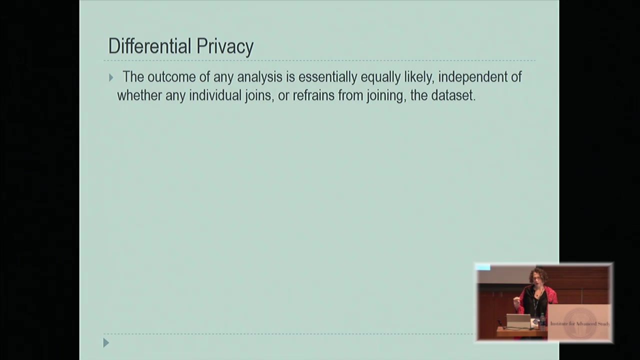 individual, For example. actually let me wait on that for a second, Okay. Okay, So we're not saying that we haven't learned something that can be used against them, And you'll see an example in a minute. But the English language definition of differential privacy says that the outcome of any analysis 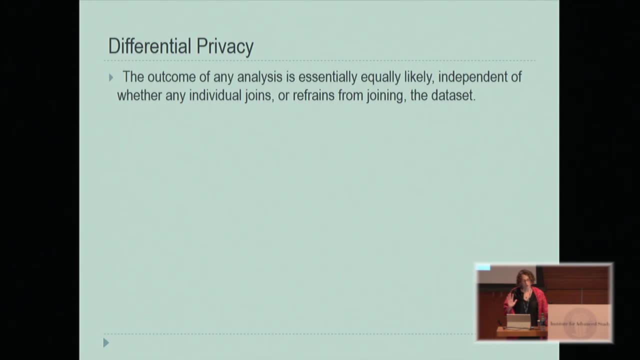 is essentially equally likely, independent of whether any individual joins or refrains from joining the data set. So we'll learn essentially the same things with essentially the same probabilities. if Nissenbaum goes away, If Sweeney joins, Nissenbaum is replaced by Sweeney and other small changes to the data set. Now 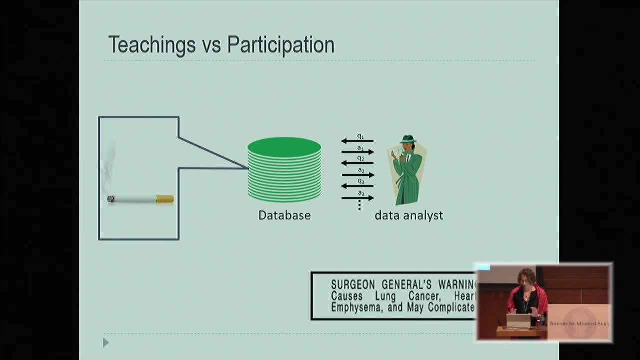 as I said, differential privacy separates the harms that could come from the teachings of the database from the harms that can come from participation. So suppose the data set teaches us that smoking causes cancer and it's known that somebody smokes, this person's insurance premiums may rise. they've been 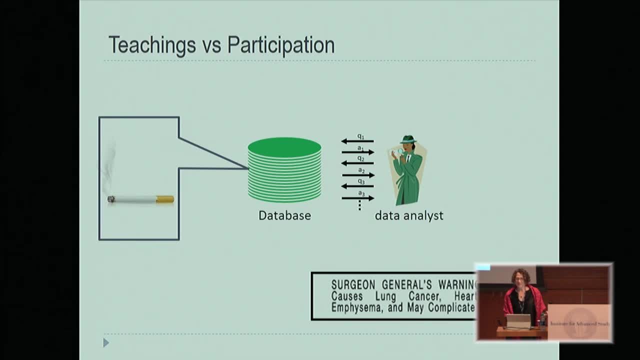 harmed by the teachings of the data set. but they would be harmed in this way and the premiums would rise, independent of whether that particular smoker is in the data set or out of the data set. and learning that smoking causes cancer is the whole point of statistical data analysis and in fact the smoker can also. 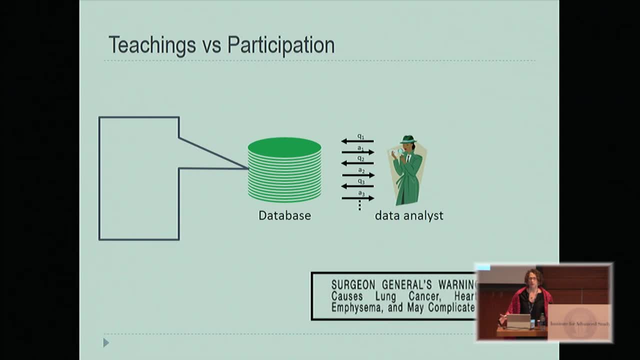 be Потому否这个信息被人用来指使有无否中心选字的话, officers, ads, and in fact the smoker can also be helped because, having learned this, the smoker can now choose to join a smoking cessation program. maybe you know inspired to join a smoking cessation. 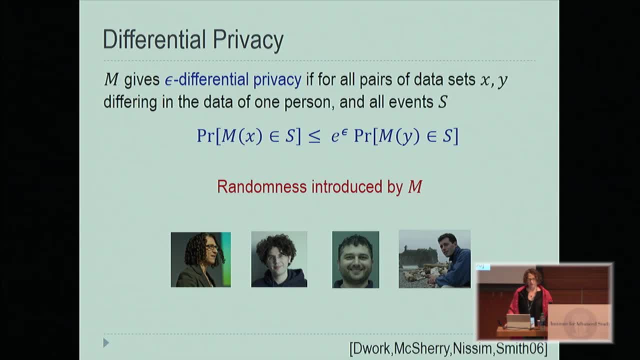 program. So here's the formal definition of differential privacy. First of all, we need the concept of data sets that differ in the data of one person: adjacent data sets. So adjacent data sets are data sets that are almost identical, but one is slightly smaller than the other, and the larger one contains the 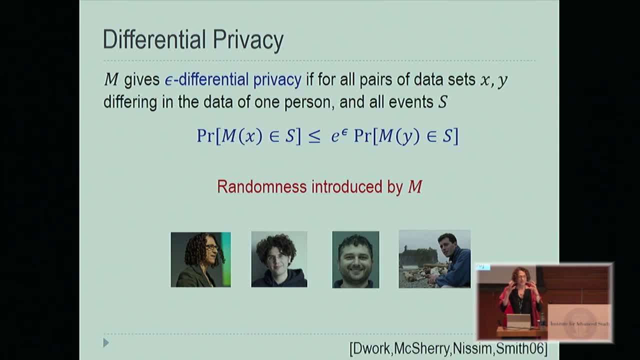 data of just one more person. So, for example, the data of everybody in this room and the data of everybody in this room except Nissenbaum. Those are two adjacent or neighboring data sets. Our algorithms that will analyze data sets will flip coins, They'll be randomized algorithms And there is a parameter. 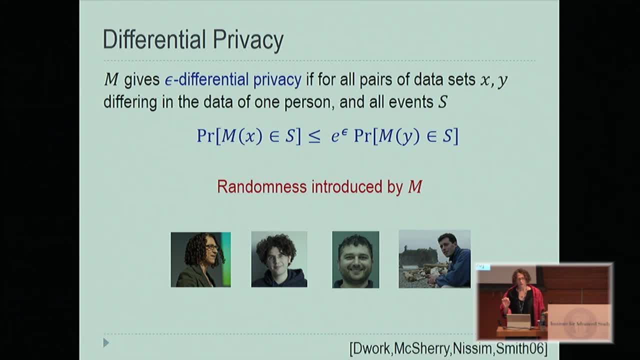 epsilon, whose role you'll see in a second. So our algorithm or mechanism M gives epsilon differential privacy. if for all pairs of data sets X and Y that differ in the data of just one person, so the data with Helen and without Helen and every possible output event S the probability that we see, S when the data 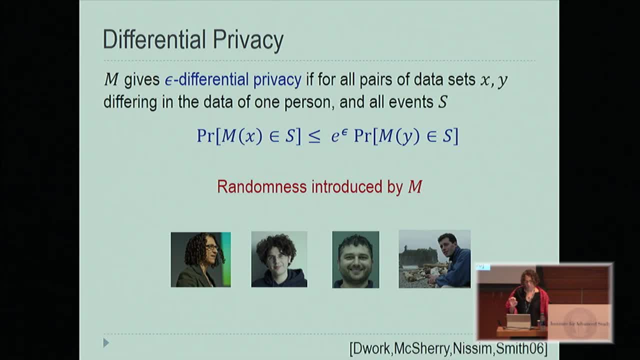 set is X is almost the same as it's, at most e to the epsilon times, the probability that we see X. when the data set is X is almost the same as it's, at most e to the epsilon times, the probability that we see. 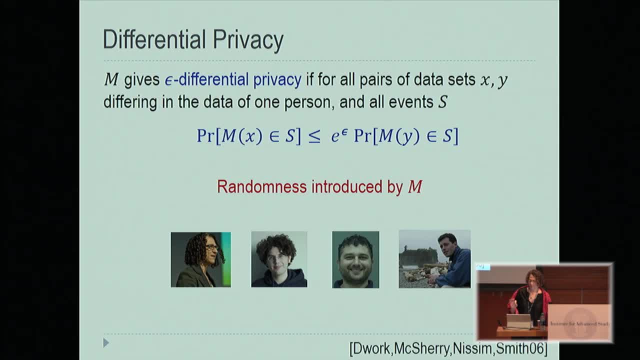 S when the data set is Y. So the ratio of those two probabilities is, at most e to the epsilon, And the probability space is over the coin flips of the algorithm. The algorithm is the good guy. So, arbitrary data sets, the algorithm is the good guy. 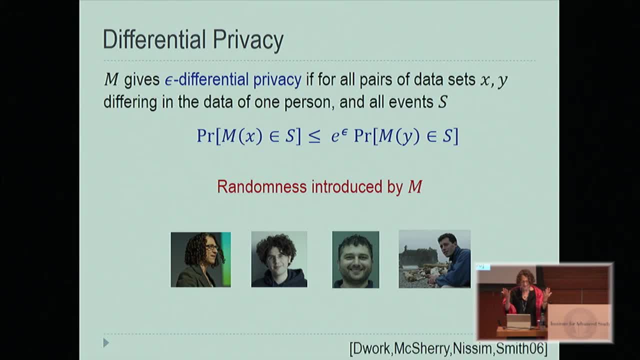 And because we said for all pairs of data sets, the same inequality would hold if we swap the roles of X and Y. So this is a definition that was put forward by, together with McSherry, Nisim and Smith in 2006.. 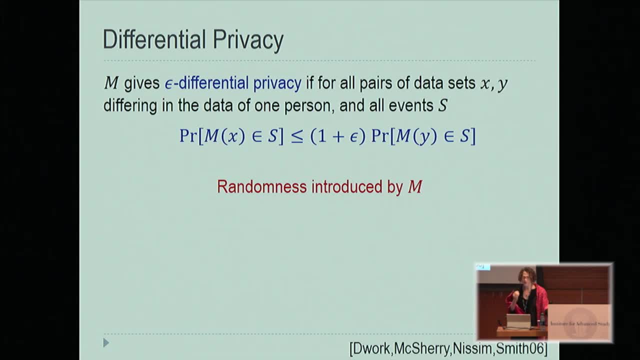 So, as you know, e to the epsilon, when epsilon is small, is about 1 plus epsilon, And this is a nice way to read this. So when epsilon is 0, it says that these two probabilities have to be the same. So when you have zero probability, loss you. 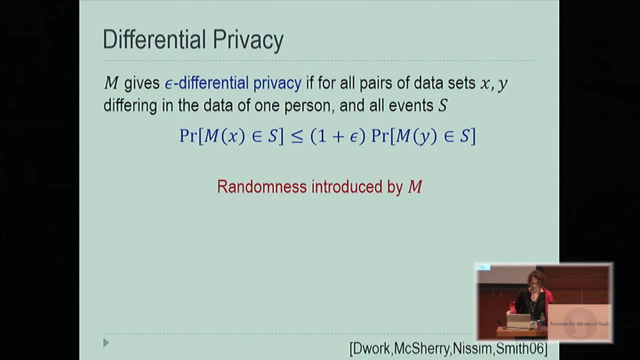 also get zero information about the data set by some kind of composition there. But when epsilon is small, this could be a very reasonable notion, And the key point is that if a bad event is very unlikely when I'm not in the data set, then it will still. 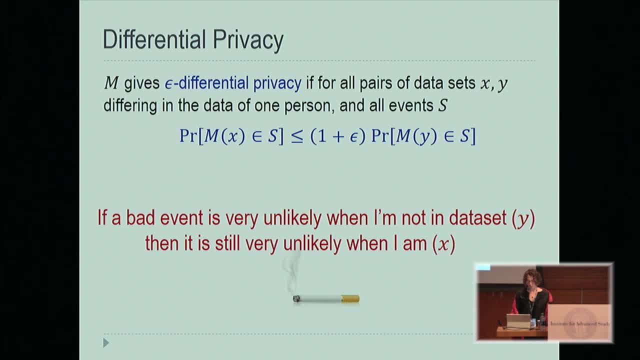 be very unlikely when I am in the data set. So, for example, if I'm going to be charged higher premiums when- I'm sorry I shouldn't have used that example- If I'm going to be identified as a member of a genome-wide association study, it's going to be about 0.3 to 0.7.. 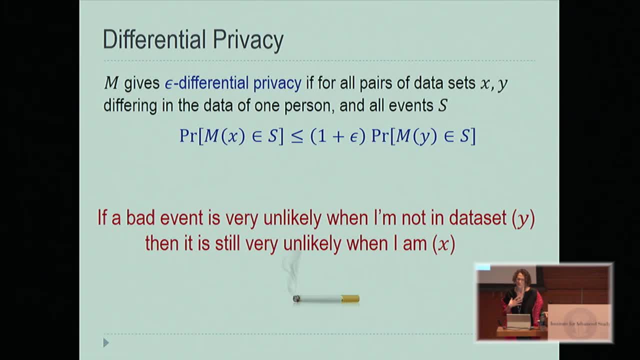 That's the likelihood, But this is really all about the probability, because we're talking study case group when – I can't be identified as a member of a genome-wide association study when I'm not actually in the study. Therefore, if I am in the study, then still I will be very unlikely – in fact zero. 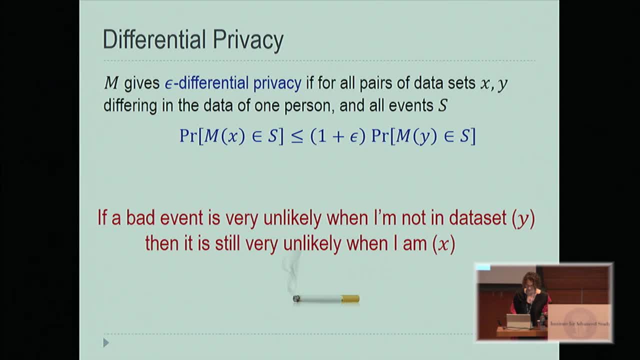 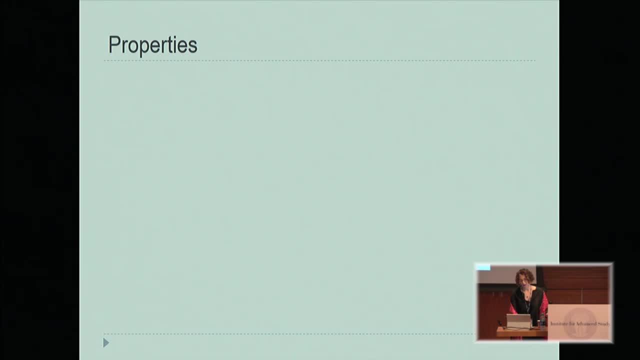 probability of being identified as a member of the case group. So epsilon is our measure of privacy loss. Now there are some properties of differentially private algorithms that flow directly from the definition, independent of the actual implementation, of the actual algorithm. that's achieving differential privacy. 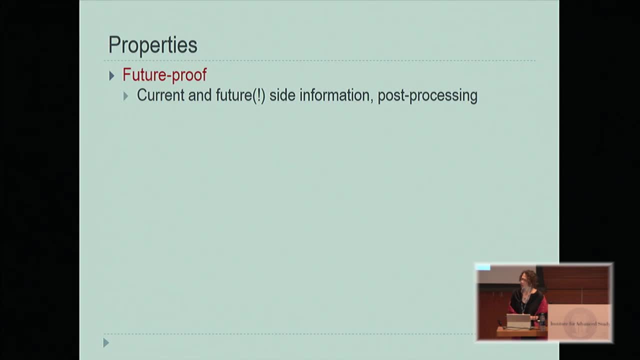 First of all, differentially private algorithms are future-proof. Privacy comes from the process by which the outputs are generated, and if a data release is differentially private, That ratio of probabilities doesn't change. if somebody who sees the output goes off and learns other auxiliary information or sees other data sets, that will exist not even now. 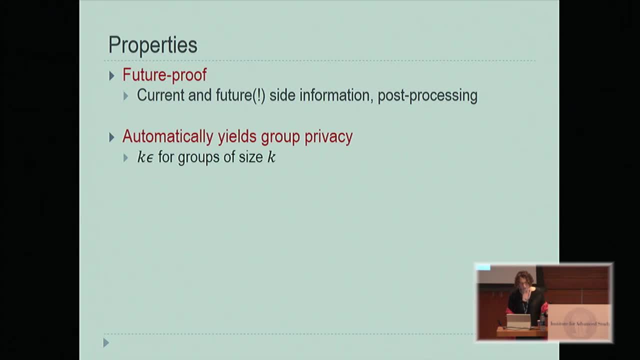 but in the future, If an algorithm yields epsilon differential privacy for a single individual, then it automatically yields k epsilon differential privacy for groups of size k. So if you're happy with epsilon differential privacy for you and you have a family of size 5, you'll see that your family has privacy of 5 epsilon and you can decide how you feel. 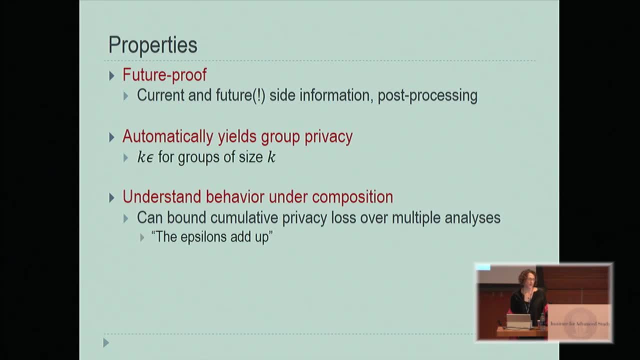 about that. Most importantly is that we can understand the behavior of privacy loss, of differential privacy under composition. That is to say, we can bound the cumulative privacy loss. We can bound the cumulative privacy loss over multiple analyses. One crude bound shows us that in the worst case the epsilons add up. 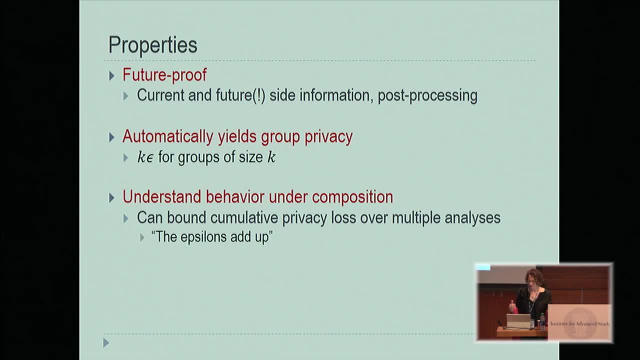 We can do better than that, and that will be the subject of Guy Rothblum's talk. He's going to talk about composition Because of the composition property, which says that we can understand when we ask about many different statistics, We get that differentially private algorithms are actually programmable. 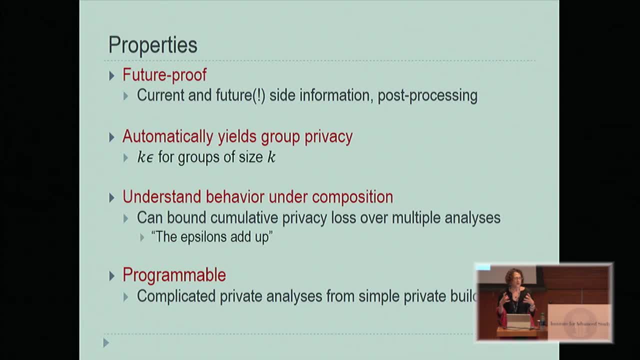 That is to say, in ordinary programming you don't just compute everything from ands and ors, even though you guys probably know that anything that you can compute can be computed just using ands and ors. What we do is we build little subroutines and algorithms for smaller problems and the 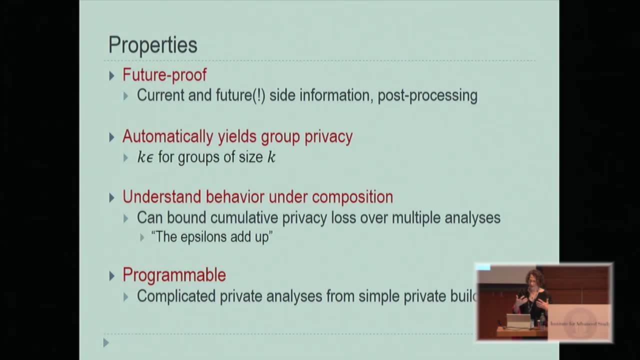 whole field of algorithm design is the curriculum, So we can build algorithms for smaller problems. and the whole field of algorithm design is the curriculum. It's a creative and intelligent combination of different computational building blocks to carry out a sophisticated computational task while minimizing some sorts of resources. 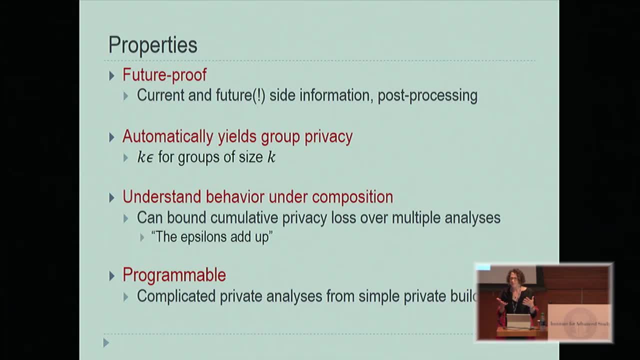 like time or space. The same thing is true with differential privacy. You can take small, differentially private building blocks and combine them to carry out complex, differentially private data analyses, and that is a power that none of the other approaches have, as far as I know. 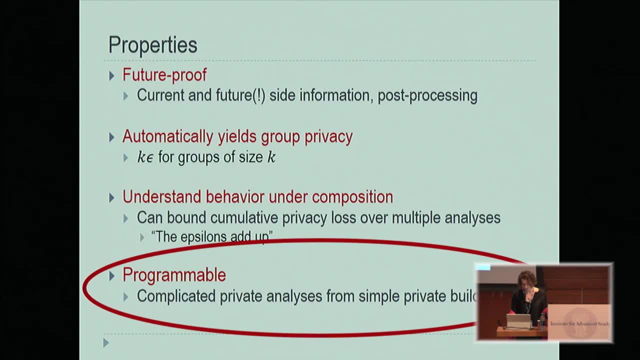 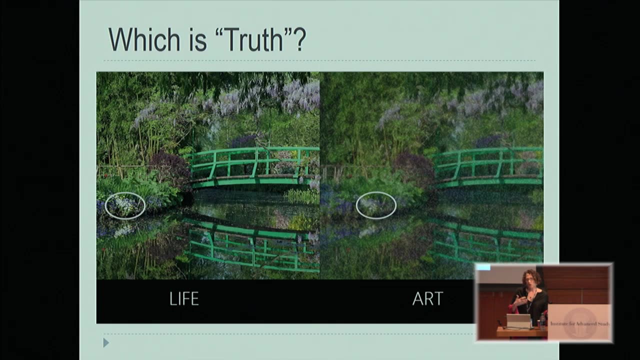 And that is going to be the subject of Kunal Talwar's talk. So I've said that overly accurate estimates of too many statistics compromises privacy. So differential privacy has to somehow blur your answers a little bit, And so you have sort of truth and you have the blurred version of truth. And well, which?